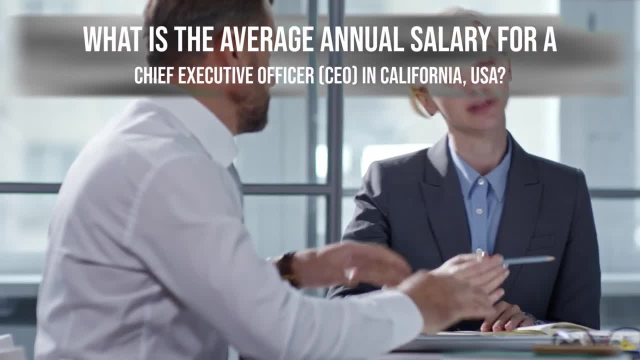 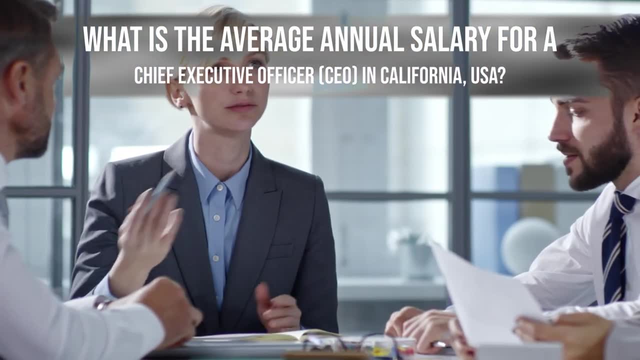 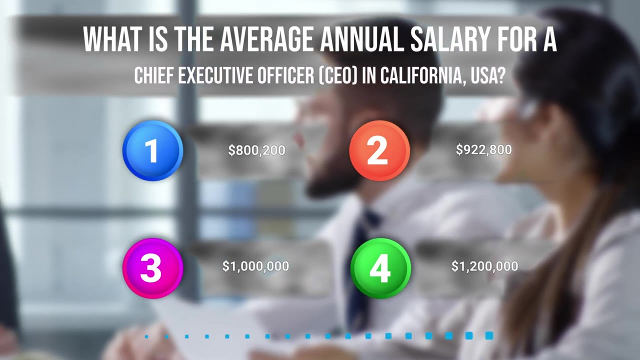 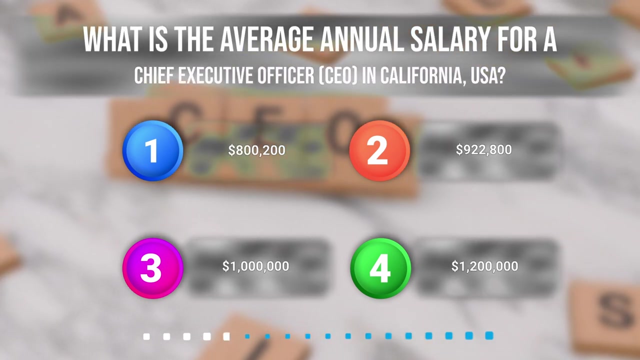 This data is as of April 2024 and sourced from the public website salarycom. What is the average annual salary for a chief executive officer in California, USA? 1. $800,200, 2. $922,800, 3. $1,000,000, 4. $1,200,000. 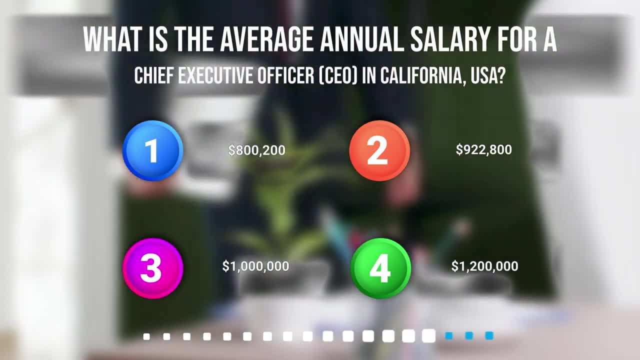 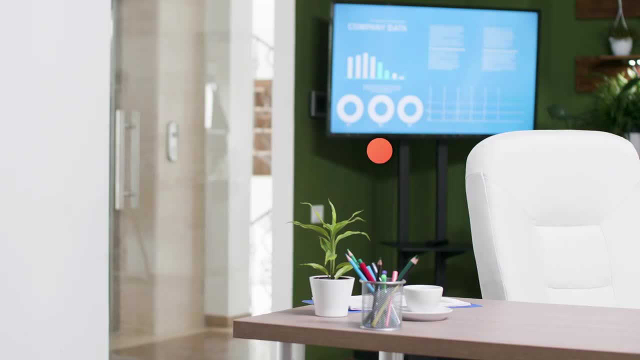 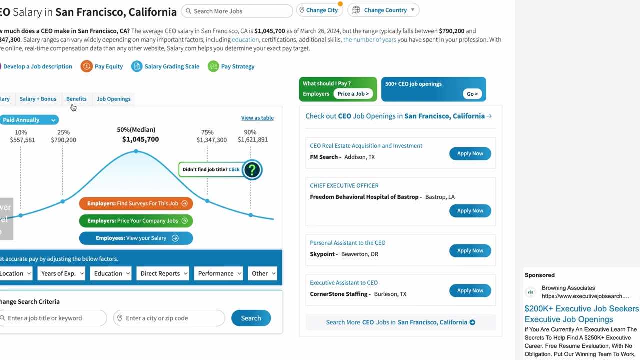 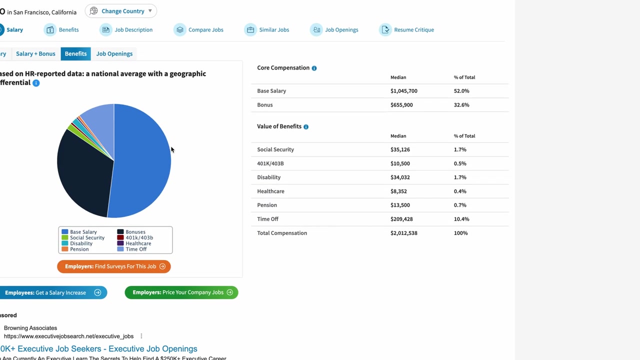 3. $150,000. 4. $1,000,000? The answer is 2. $922,800.. The average annual salary for a CEO in San Francisco, California, is $1,045,700.. The total compensation, including all the benefits: 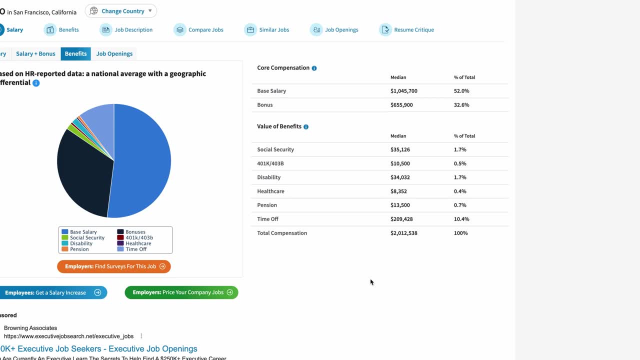 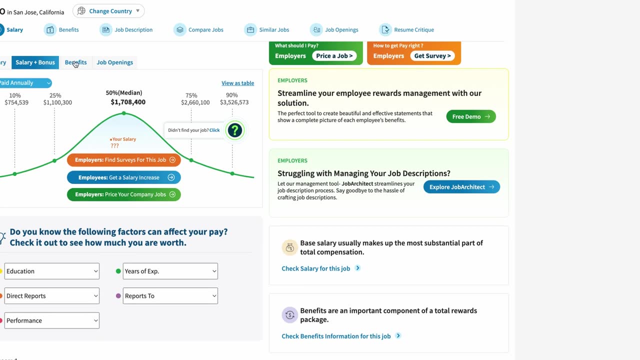 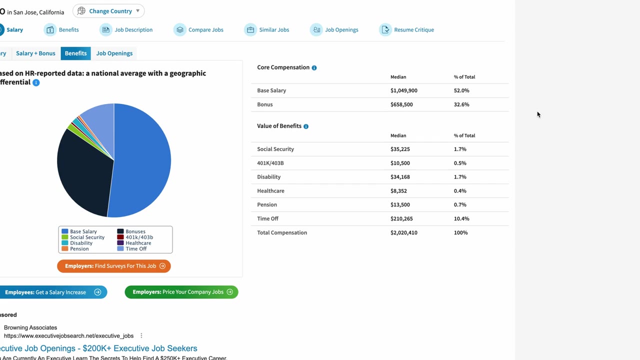 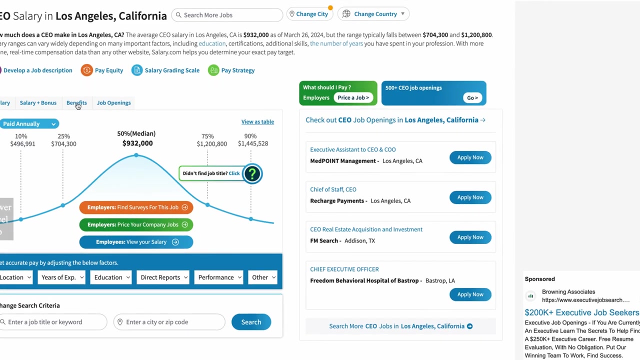 are 2,012,000.. five hundred thirty eight dollars. the average annual salary for a ceo in san jose, california, is one million forty nine thousand nine hundred dollars. the total compensation, including all the benefits, are two million twenty thousand four hundred ten dollars. the average annual salary for a ceo in los angeles, california, is nine hundred thirty two. 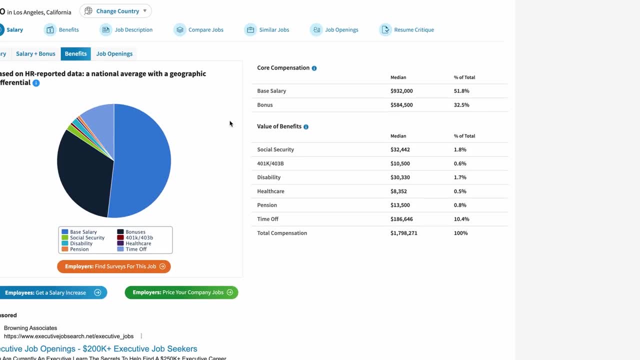 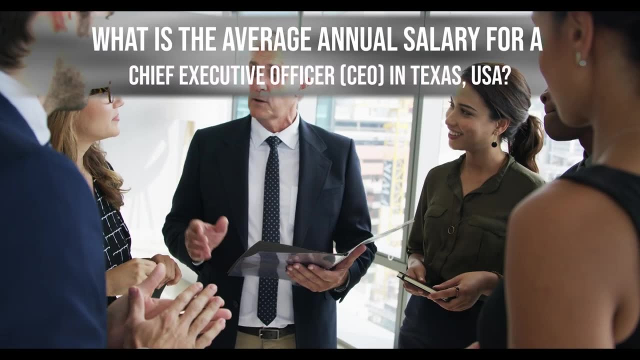 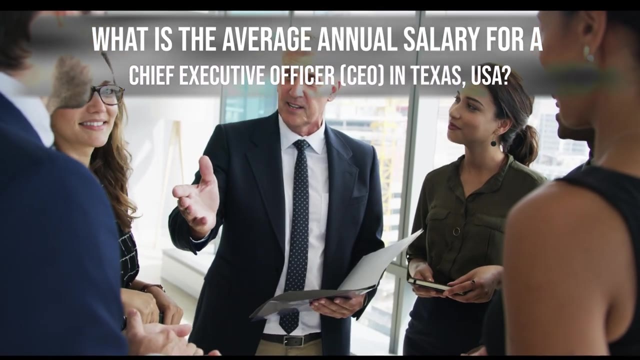 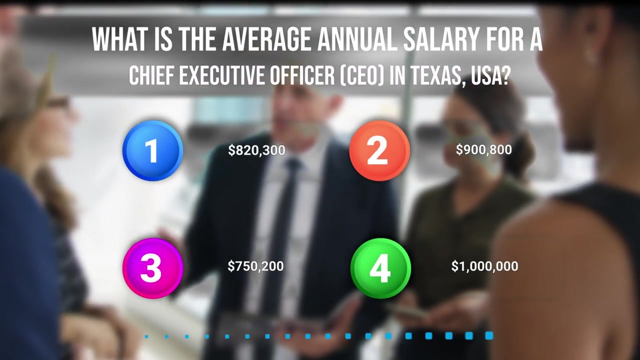 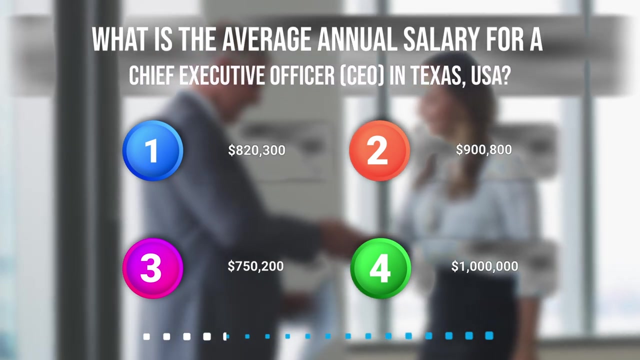 thousand dollars. the total compensation, including all the benefits, are one million seven hundred ninety eight thousand two hundred seventy one dollars. what is the average annual salary for a chief executive officer in texas, usa? one eight hundred twenty thousand three hundred dollars. two nine hundred thousand eight hundred dollars. three, seven hundred and fifty thousand two hundred dollars. four one million. 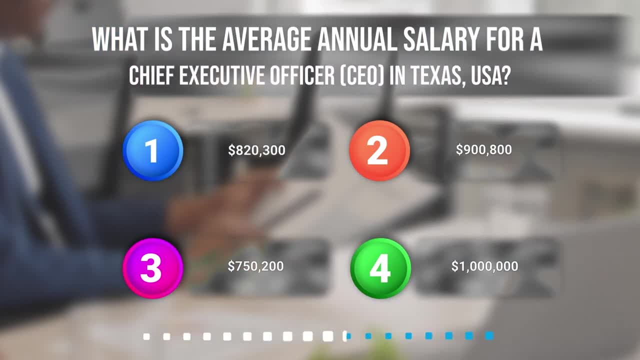 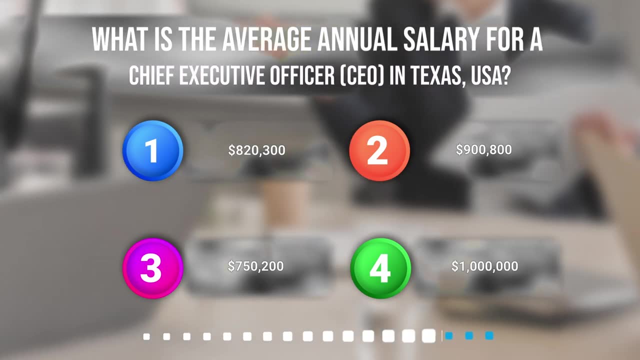 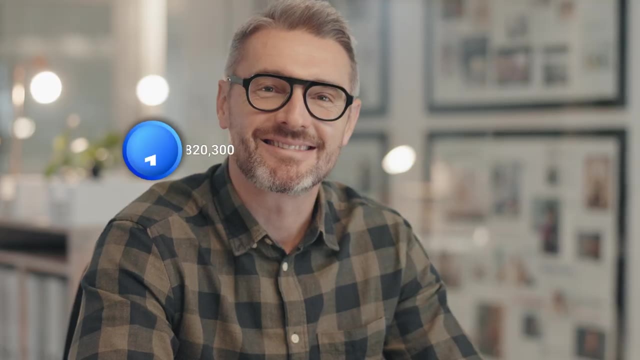 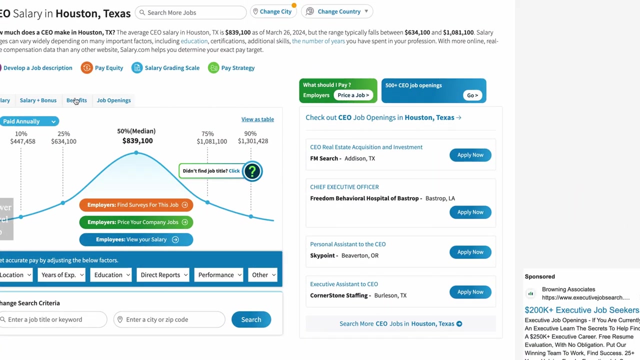 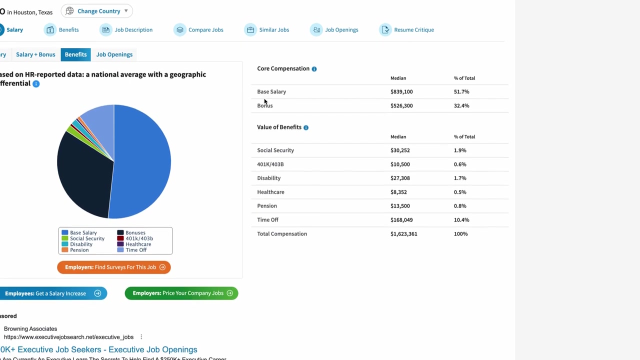 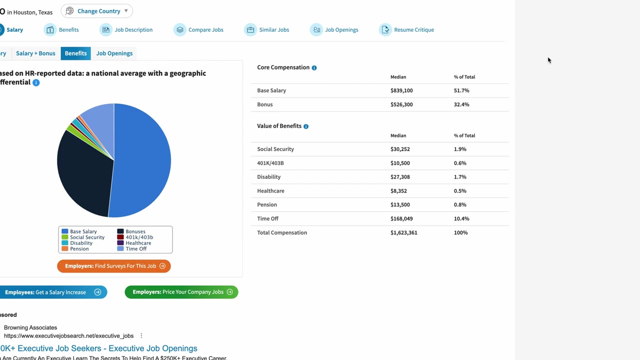 dollars. the answer is one eight hundred twenty thousand three hundred dollars. the average annual salary for a ceo in houston, texas, is eight hundred thirty nine thousand one hundred dollars. the total compensation, including all the benefits, are one million six hundred twenty three thousand three hundred sixty one dollars. the average annual salary for a ceo in 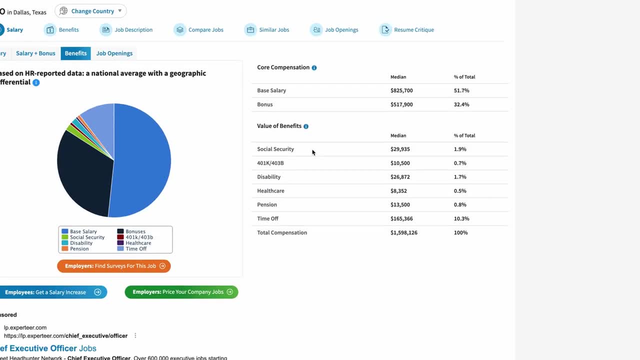 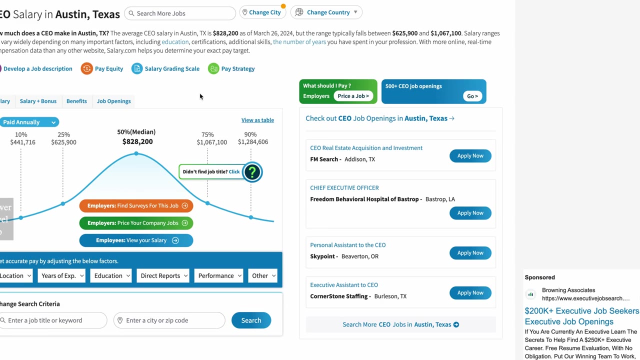 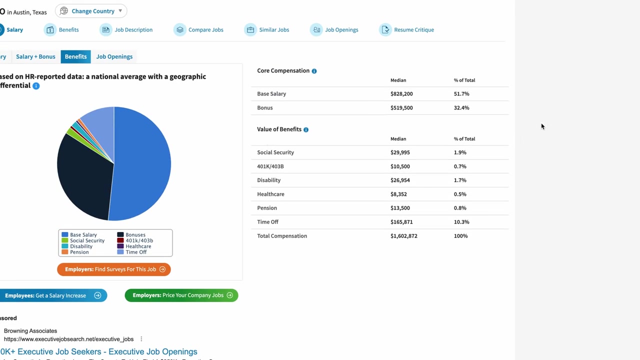 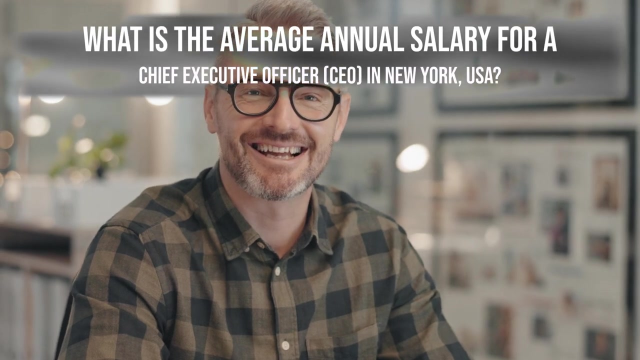 dallas, texas, is eight hundred twenty five thousand seven hundred dollars. the total compensation, including all the benefits, are one million five hundred ninety eight thousand one hundred, and The average annual salary for a CEO in Austin, Texas, is $828,200.. The total compensation, including all the benefits, are $1,602,872. 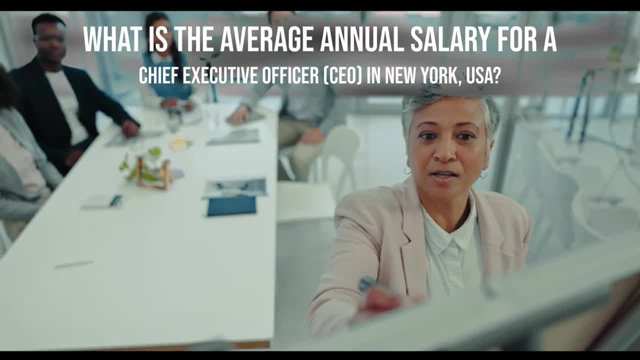 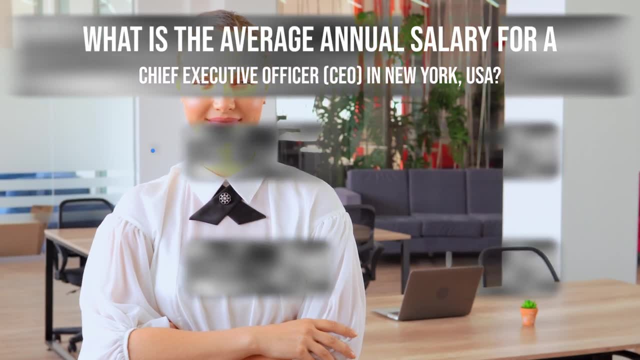 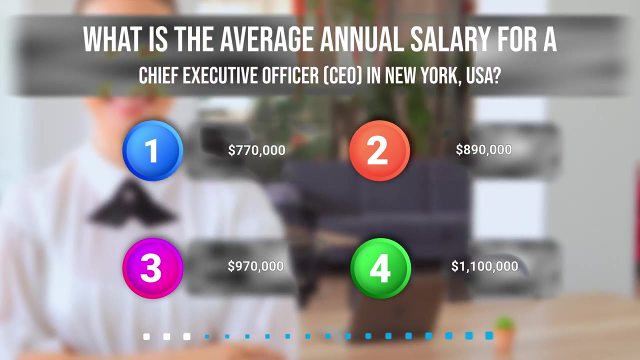 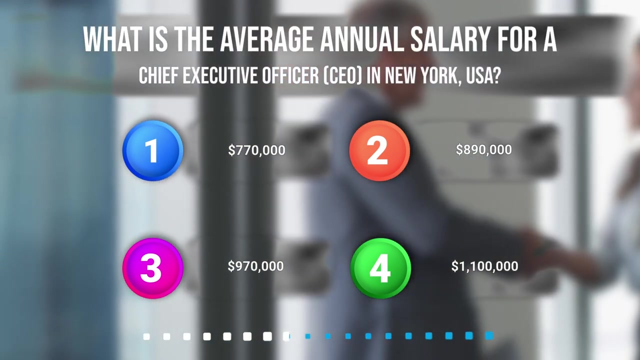 What is the average annual salary for a chief executive officer in New York USA? 1. $770,000. 2. $890,000, 3. $970,000, 4. $1,100,000. What is the average annual salary for a chief executive officer in New York USA? 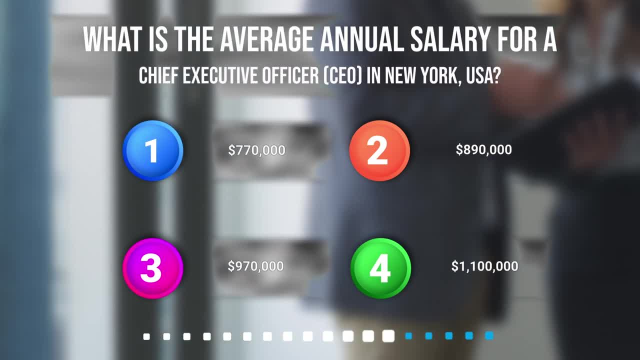 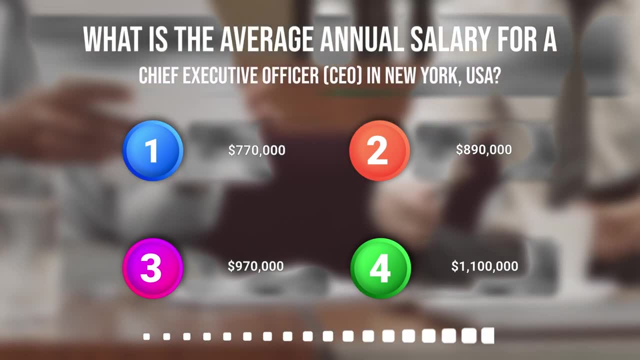 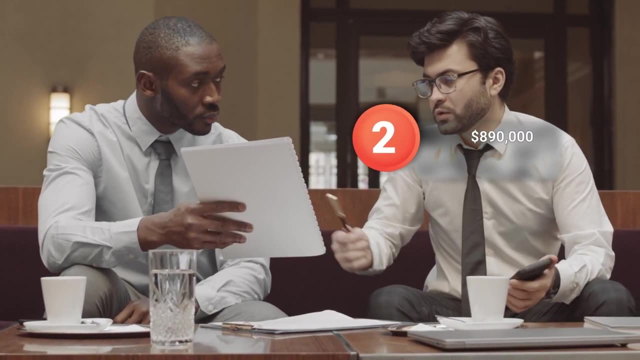 What is the average annual salary for a chief executive officer in New York USA? 1. $770,000. 2. $890,000. The answer is 2. $890,000. What is the average annual salary for a chief executive officer in New York USA? 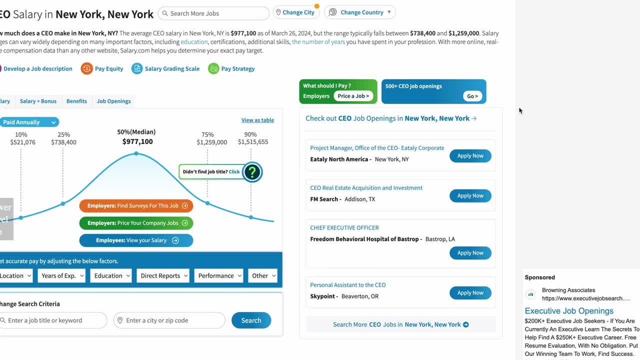 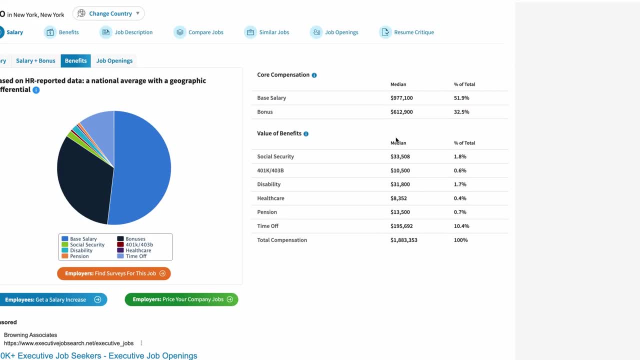 The average annual salary for a chief executive officer in New York, USA is $977,100.. The total compensation, including all the benefits, are: The average annual salary for a chief executive officer in New York, USA is $977,100.. The total compensation, including all the benefits, are: 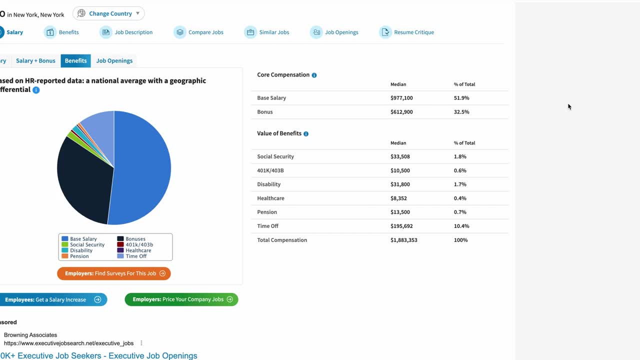 The average annual salary for a chief executive officer in New York, USA is $1,883,353.. The average annual salary for a chief executive officer in New York, USA is $959,600.. The total compensation, including all the benefits, are: The average annual salary for a chief executive officer in New York, USA is $1,883,353.. The average annual salary for a chief executive officer in New York, USA is $959,600.. The total compensation, including all the benefits, are: The average annual salary for a chief executive officer in New York USA is $1,883,353.. The total compensation, including all the benefits, are: 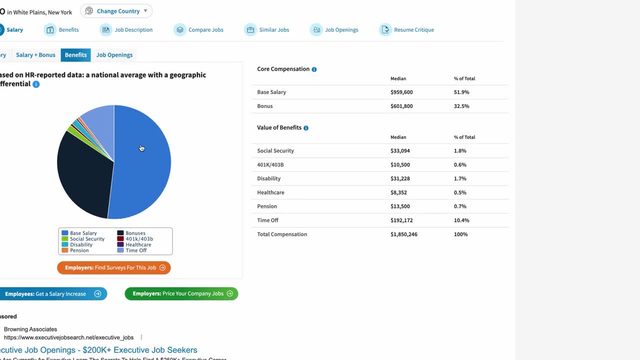 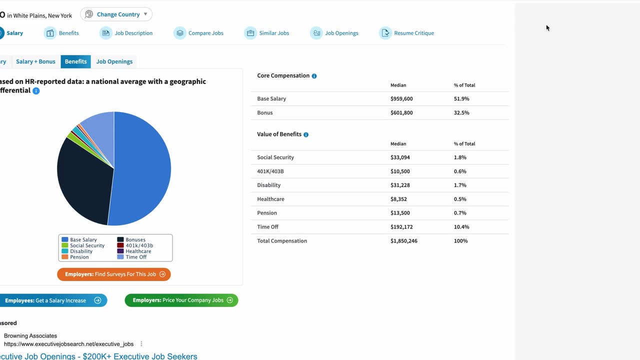 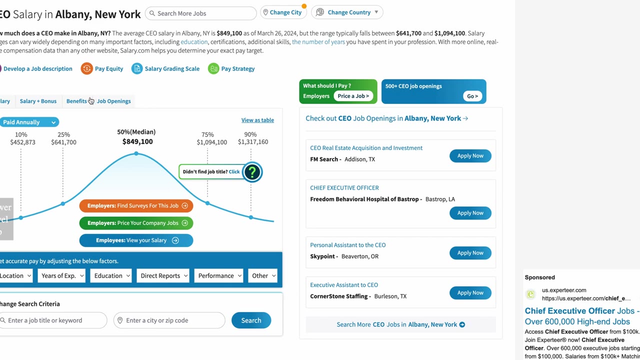 The average annual salary for a chief executive officer in New York, USA, is $959,600.. The total compensation, including all the benefits are: The total compensation including all the benefits are $1,850,246.. The average annual salary for a CEO in Albany, New York, is $849,100.. 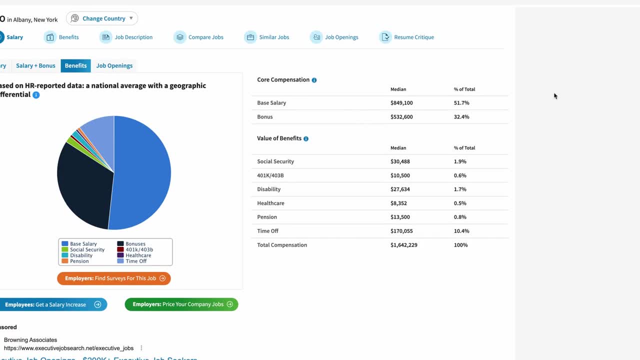 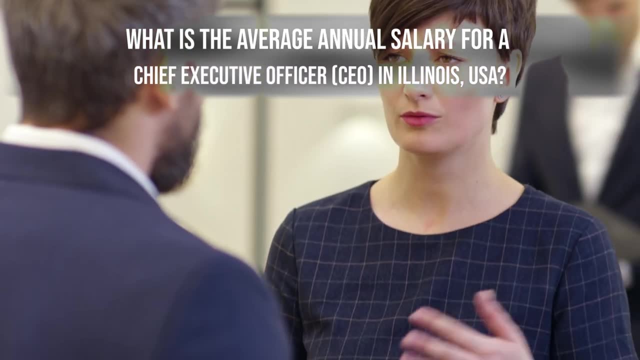 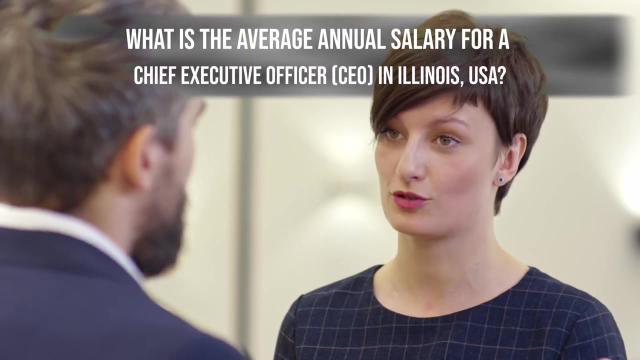 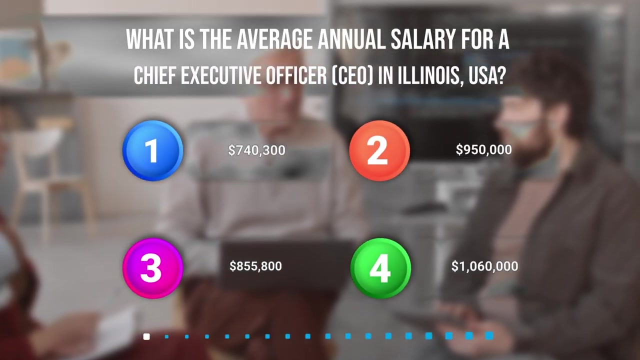 The total compensation, including all the benefits, are $1,642,229.. What is the average annual salary for a chief executive officer in Illinois, USA? 1. $740,300. 2. $950,000. 3. $855,800. 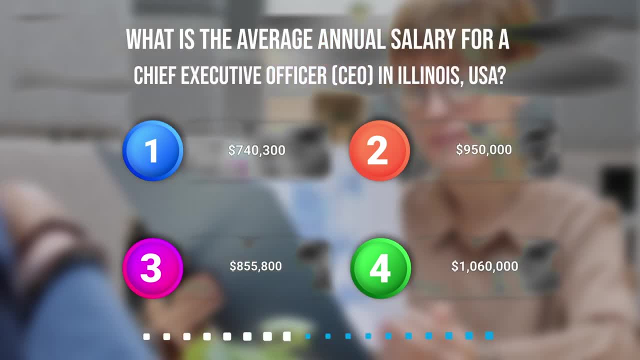 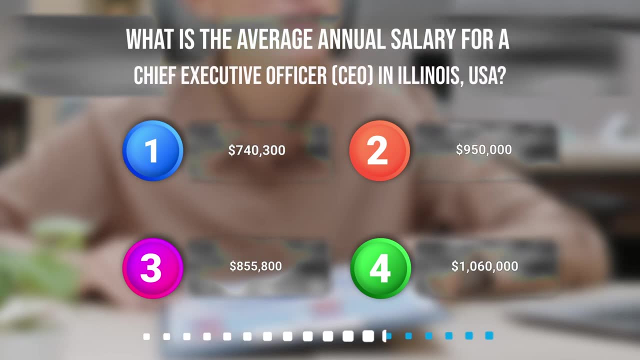 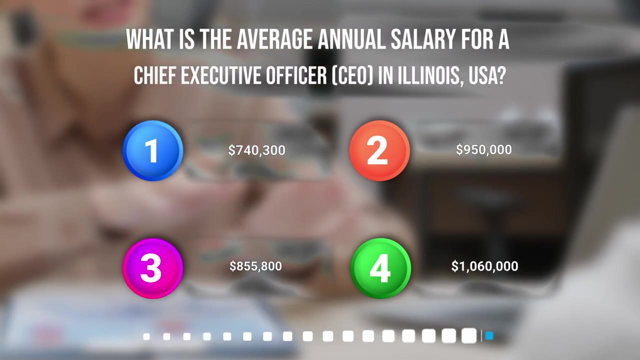 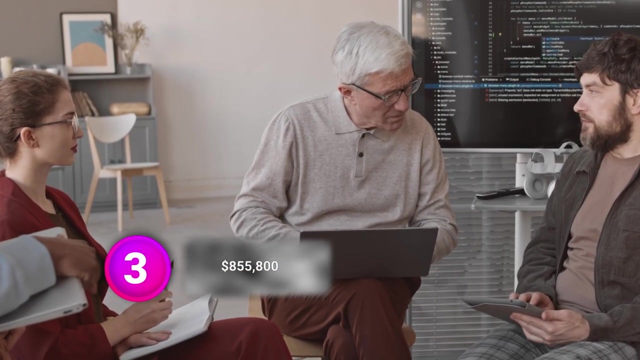 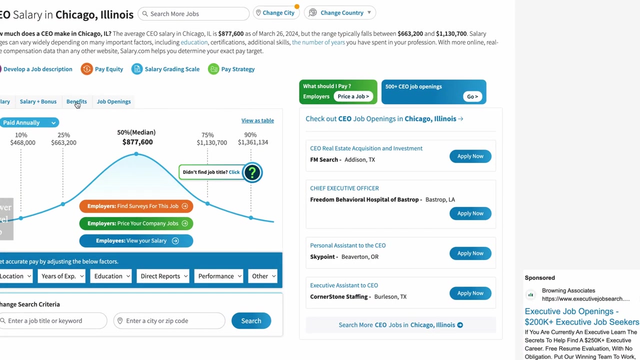 4. $1,060,000, 5. $1,000,000, 6. $1,000,000. The answer is 3. $855,800.. The average annual salary for a CEO in Chicago, Illinois, is $877,600.. 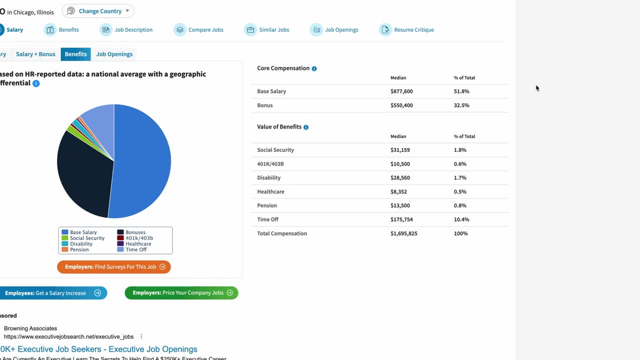 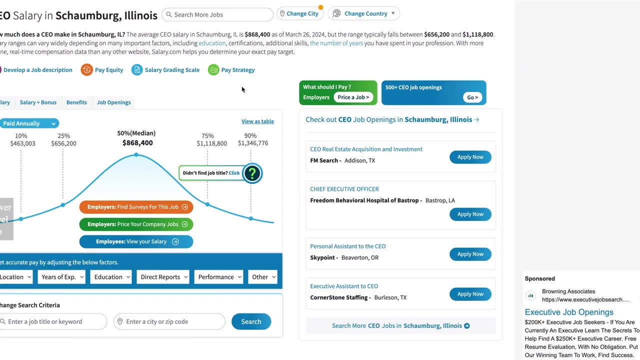 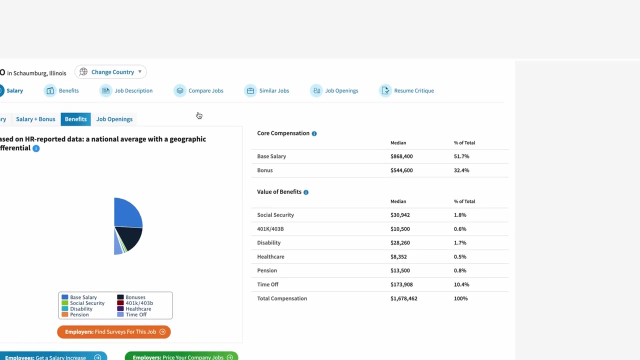 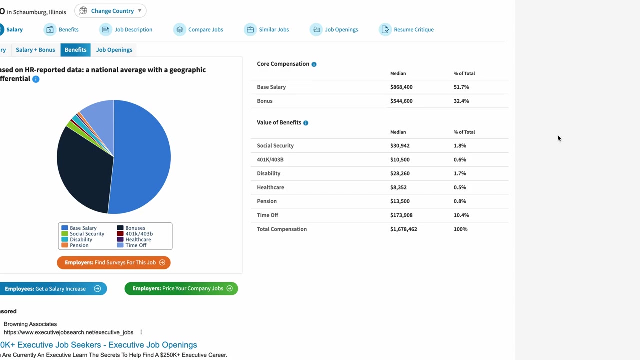 The total compensation, including all the benefits are $1,695,825.. The average annual salary for a CEO in Schaumburg, Illinois, is $868,400.. The total compensation, including all the benefits, are $1,678,462.. The answer is 3.. $1,678,462.. The average annual salary for a CEO in Chicago, Illinois, is $868,400.. The total compensation, including all the benefits, are $1,678,462.. The average annual salary for a CEO in Oak Brook, Illinois, is $875,900.. The total compensation, including all the benefits, are $1,692,700.. 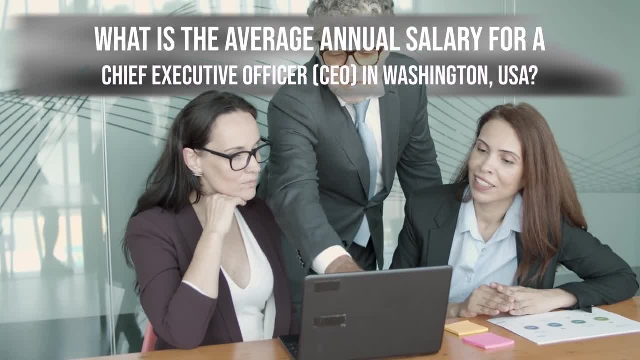 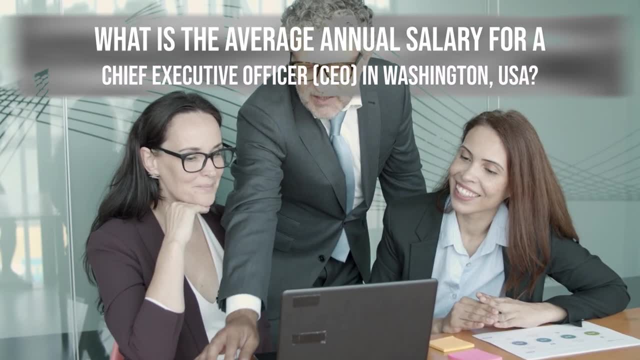 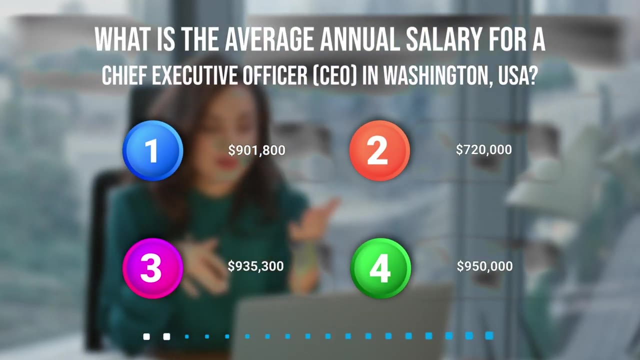 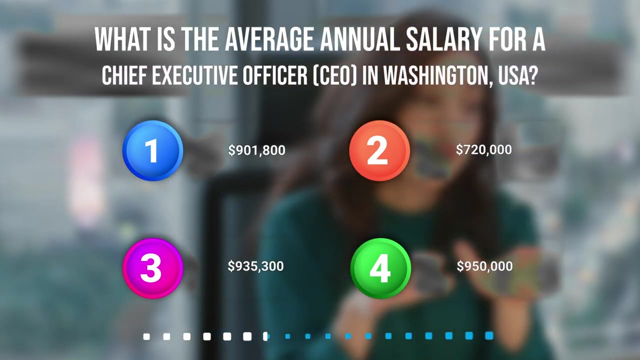 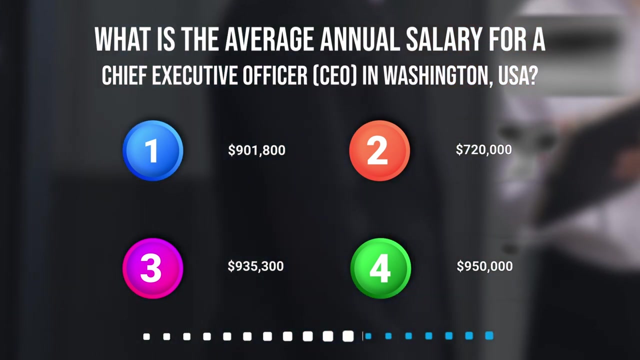 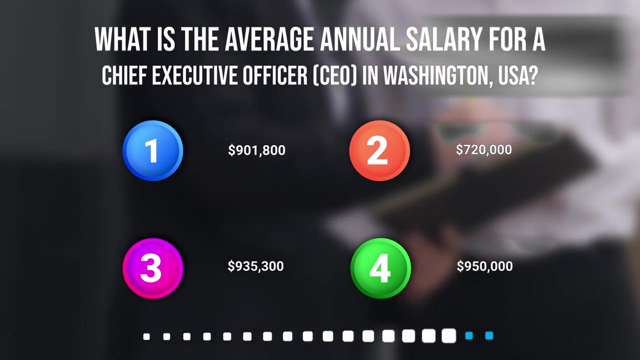 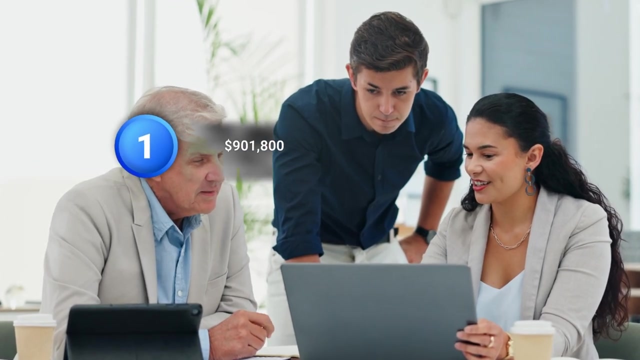 What is the average annual salary for a chief executive officer in Washington, USA? 1. $901,800. 2. $801,800, $720,000, $935,300, $950,000. The answer is 1 $901,800. 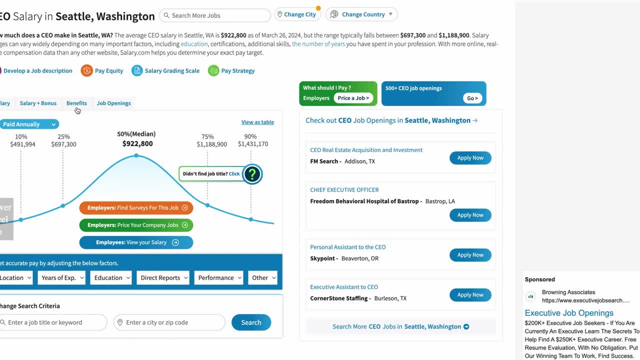 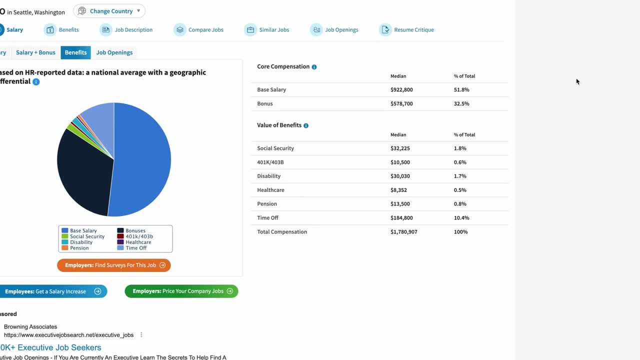 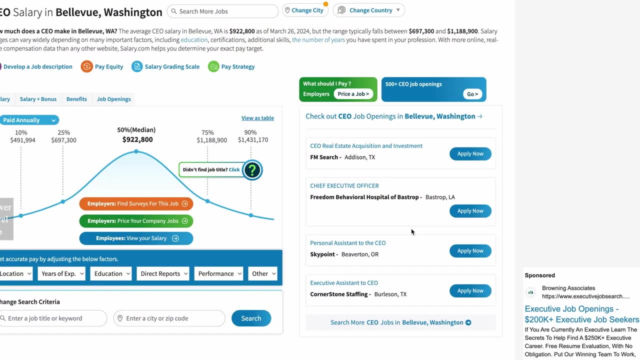 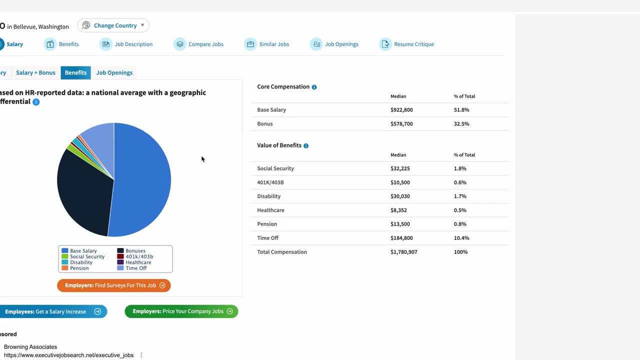 The average annual salary for a CEO in Seattle, Washington is $922,800. The total compensation including all the benefits are $1,780,907. The average annual salary for a CEO in Bellevue, Washington, is $922,800. The total compensation including all the benefits are $1,780,907. 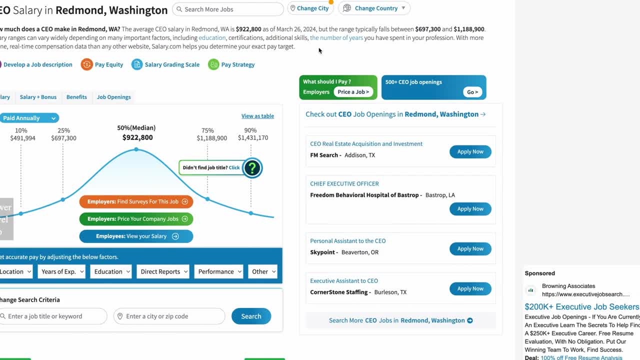 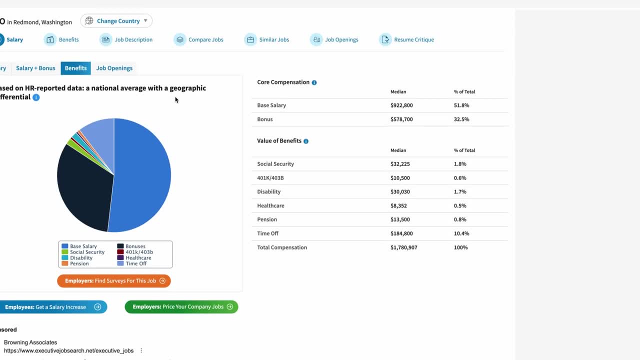 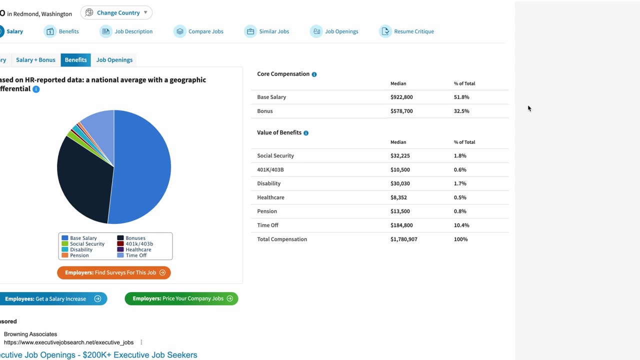 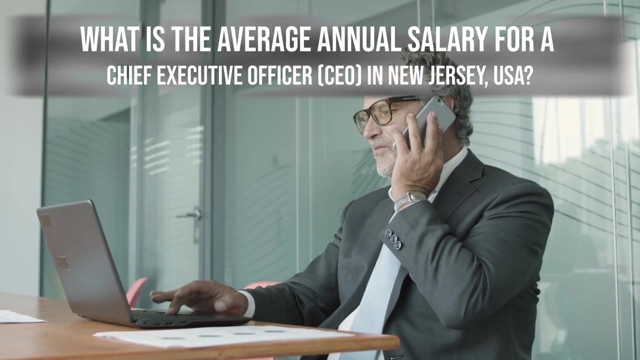 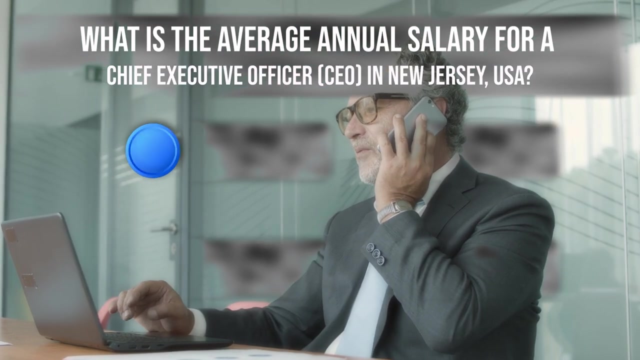 The average annual salary for a CEO in Redmond, Washington is $922,800. The total compensation, including all the benefits, are $1,780,907. What is the average annual salary for a chief executive officer in New Jersey, USA? What is the average annual salary for a chief executive officer in New Jersey, USA? 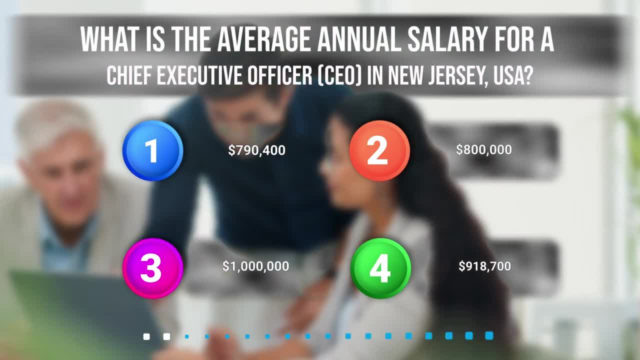 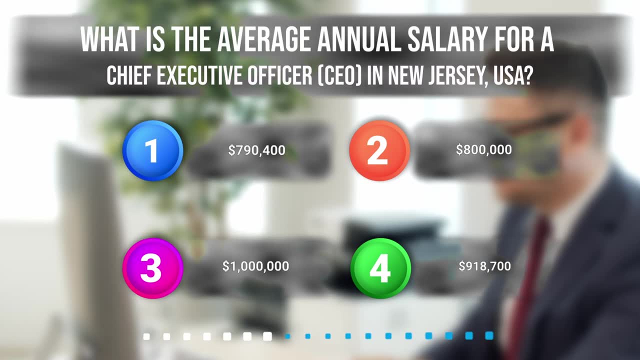 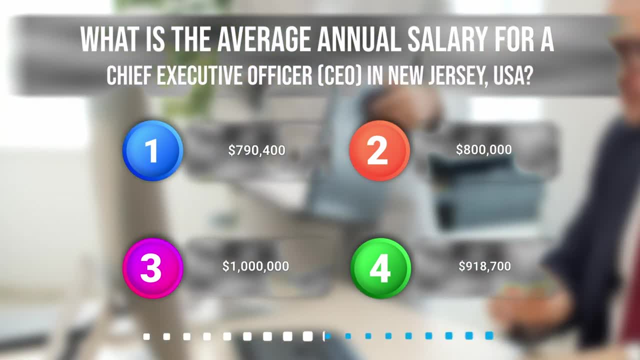 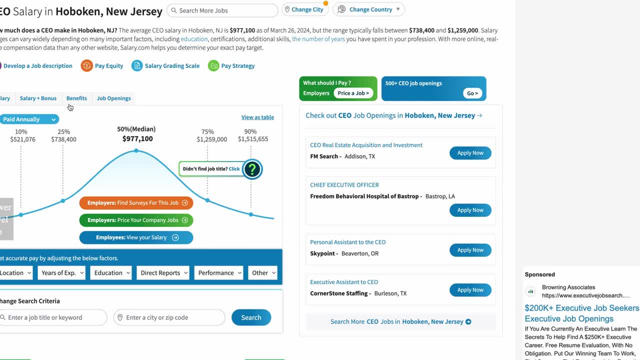 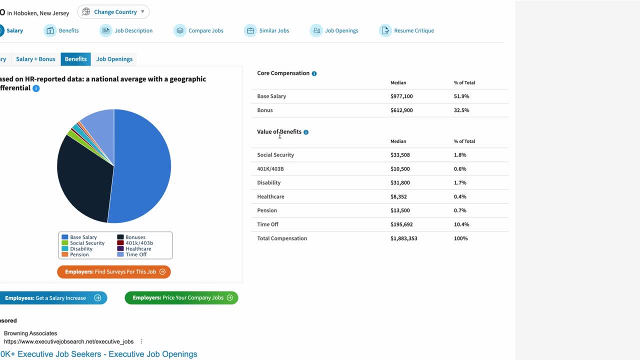 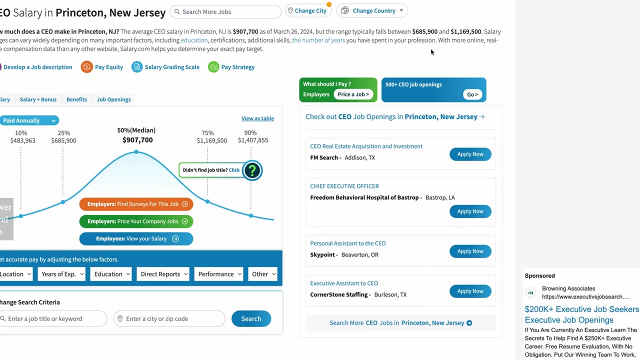 The average annual salary for a CEO in Hoboken, New Jersey, is $977,100.. The total compensation, including all the benefits, are $1,883,353.. The average annual salary for a CEO in Princeton, New Jersey, is $1,883,353. 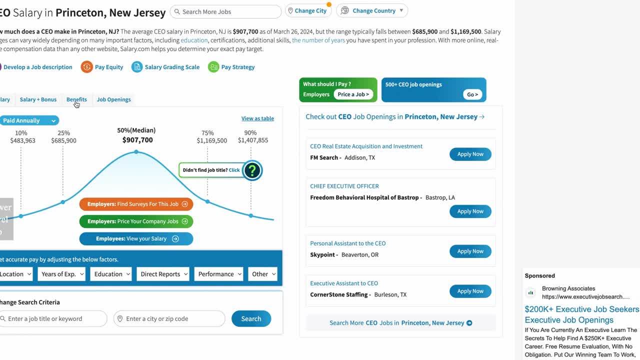 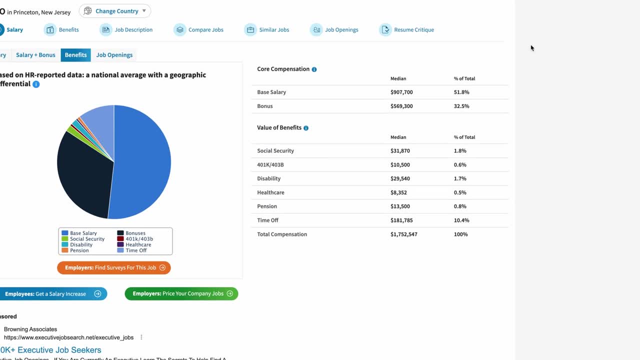 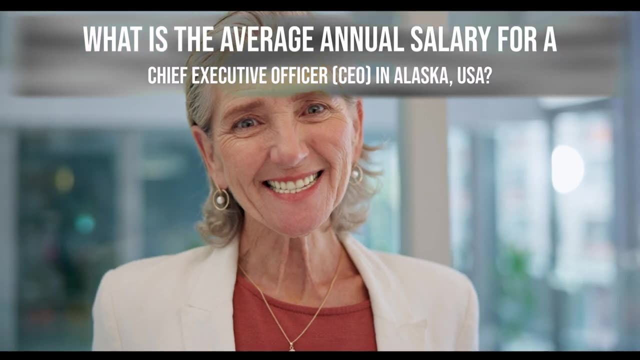 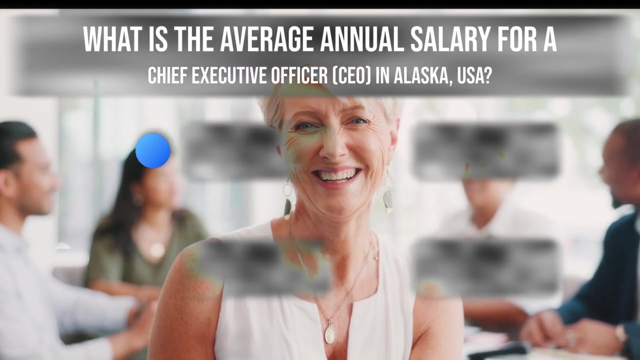 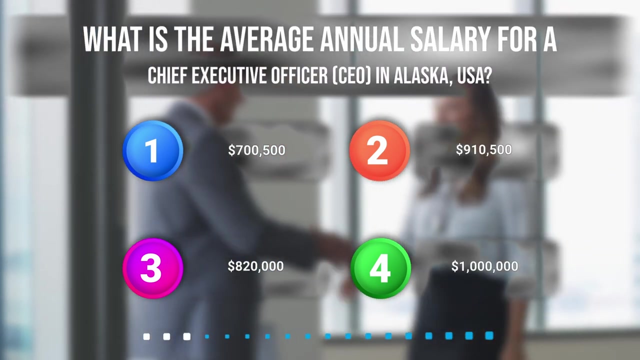 New Jersey is nine hundred seven thousand seven hundred dollars. the total compensation, including all the benefits, are one million seven hundred fifty two thousand five hundred forty seven dollars. what is the average annual salary for a chief executive officer in Alaska, USA? one seven hundred thousand five hundred dollars two. nine hundred ten thousand five hundred dollars three. 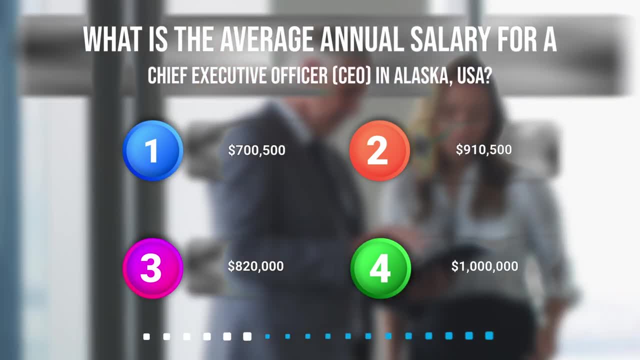 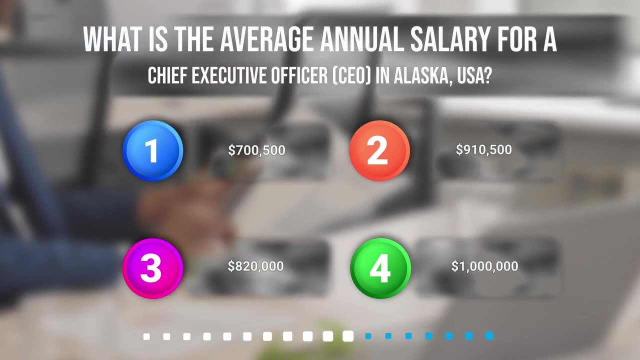 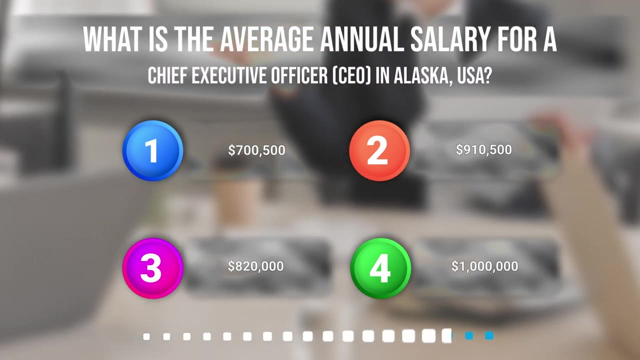 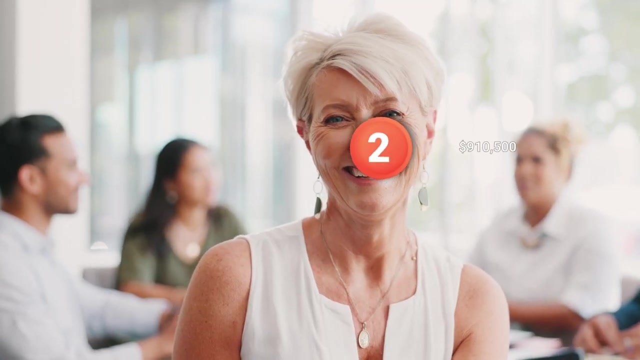 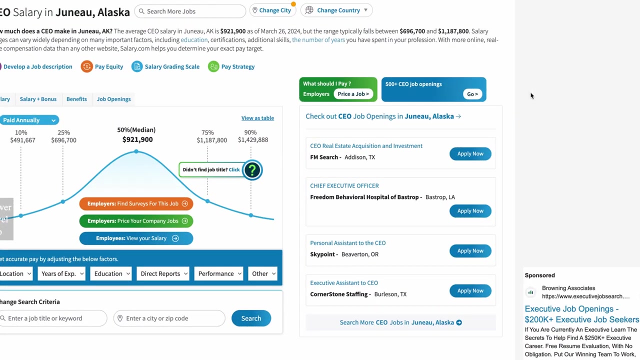 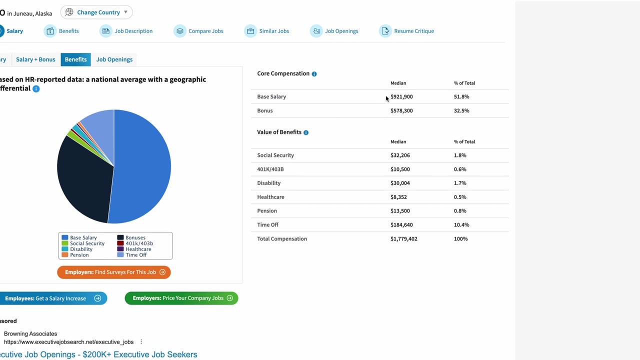 eight hundred twenty thousand dollars for one million dollars? the answer is two nine hundred five hundred fifty two nine hundred ten thousand five hundred dollars. the average annual salary for a CEO in Juneau, Alaska, is nine hundred twenty one thousand nine hundred dollars. the total compensation, including all the benefits, are one million seven hundred seventy. nine thousand four hundred two dollars. the average annual salary for a CEO in Anchorage, Alaska, is nine hundred twenty one thousand nine hundred dollars. the The total compensation, including all the benefits, are $1,779,402.. The average annual salary for a CEO in Fairbanks, Alaska, is $928,600. 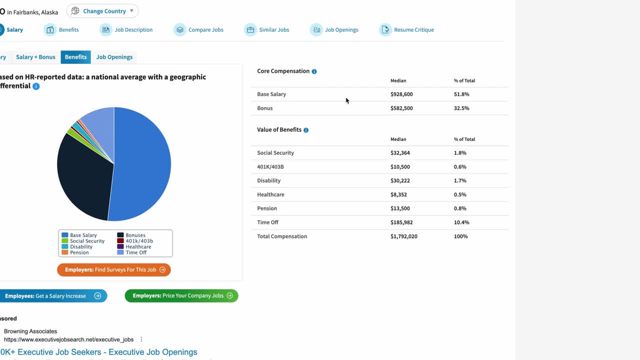 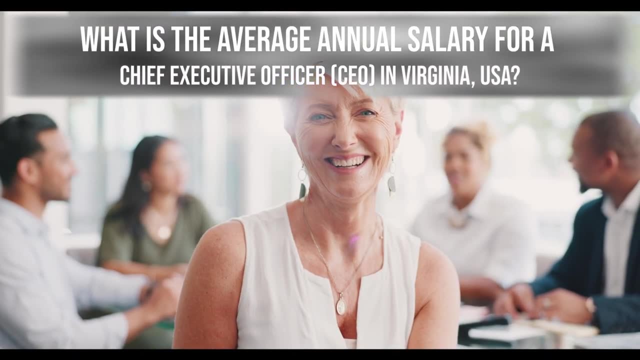 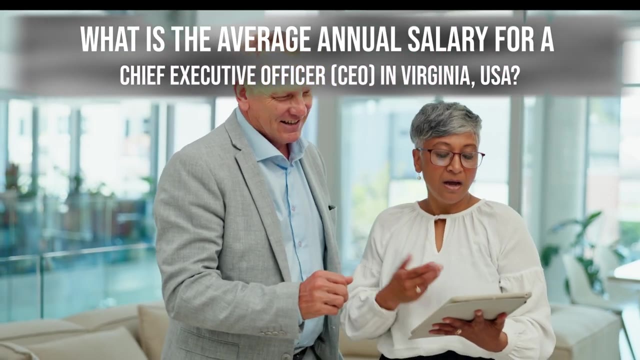 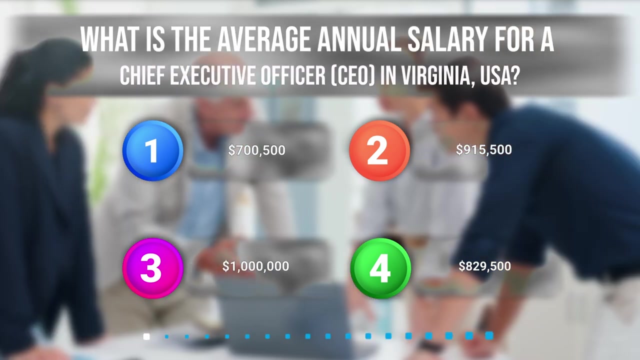 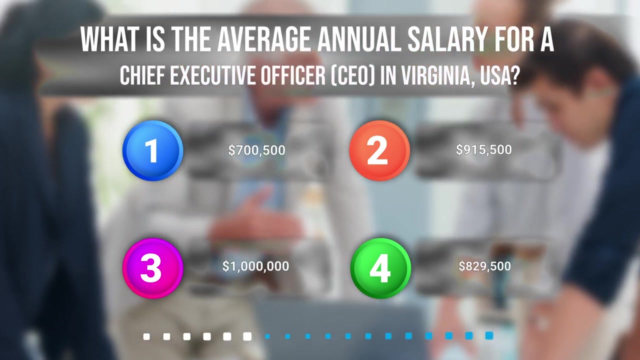 The total compensation, including all the benefits, are $1,792,020.. What is the average annual salary for a chief executive officer in Virginia, USA? $700,500, $915,500, $1,000,000, $829,500. 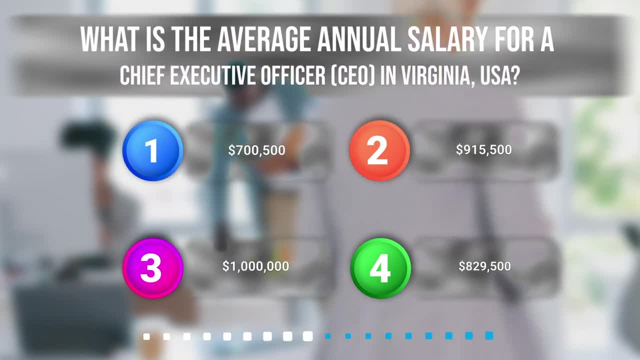 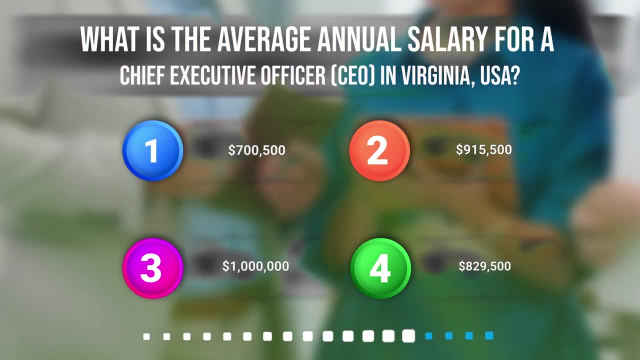 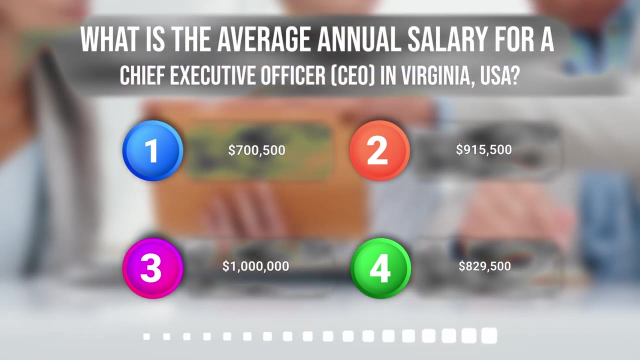 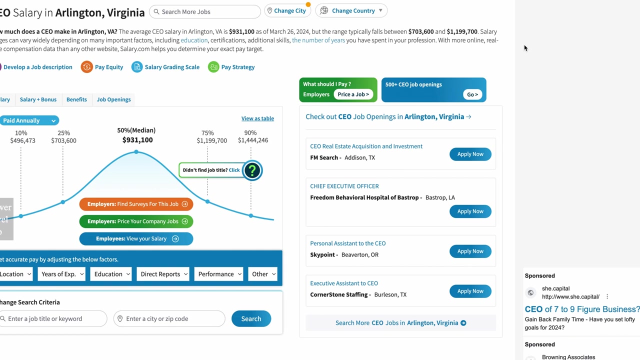 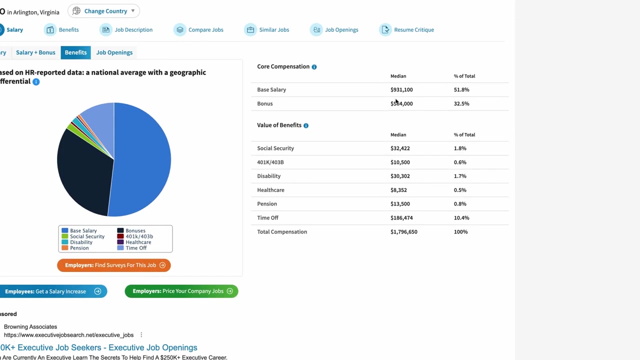 What is the average annual salary for a chief executive officer in Virginia, USA? The answer is 4, $829,500.. The average annual salary for a CEO in Arlington, Virginia, is $931,100.. The total compensation, including all the benefits, are $1,796,000. 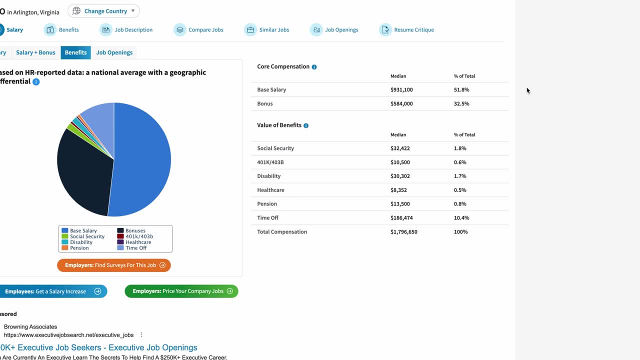 What is the average annual salary for a chief executive officer in Virginia, USA? The total compensation, including all the benefits, are $1,796,000.. What is the average annual salary for a chief executive officer in Virginia, USA? The answer is 5, $2,578,000. 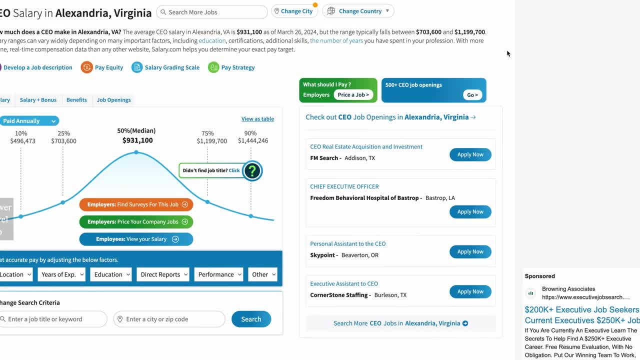 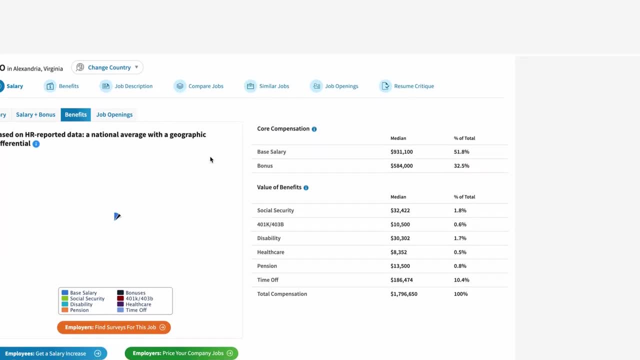 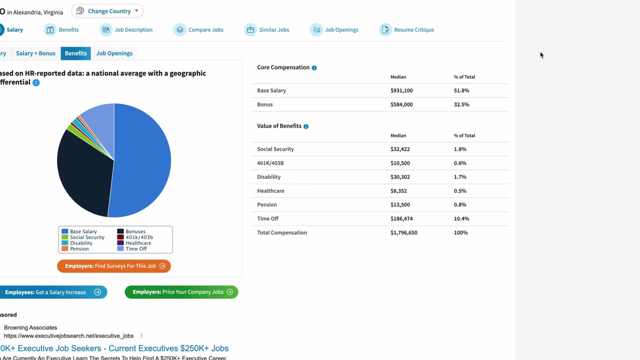 What is the average annual salary for a chief executive officer in Virginia, USA? The answer is 5, $792,000.. The total compensation, including all the benefits, are $1,796,650.. The average annual salary for a chief executive officer in Richmond, Virginia, is $814,000. 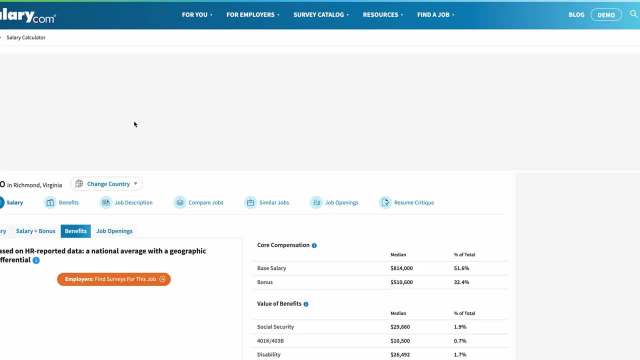 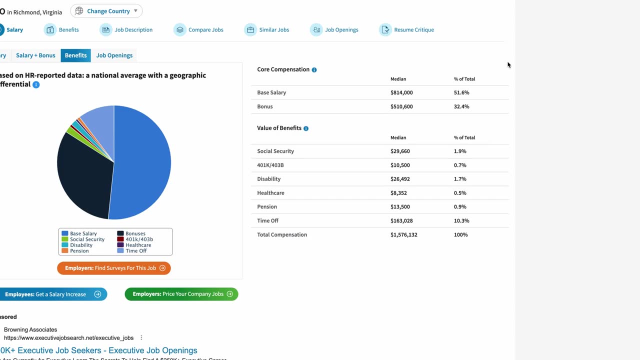 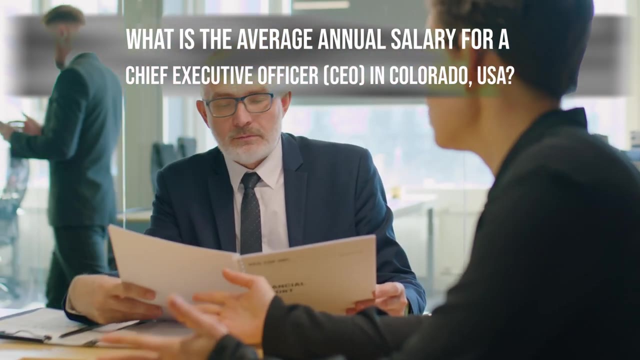 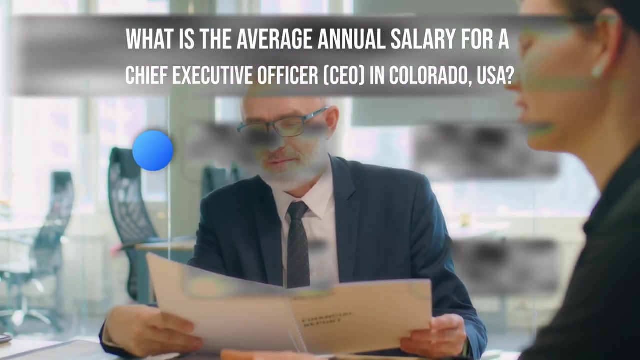 What is the average annual salary for a chief executive officer in Virginia, USA? The answer is 6, $1,776,000.. are one million five hundred seventy six thousand 132 dollars? what is the average annual salary for a chief executive officer in Colorado, USA? one. 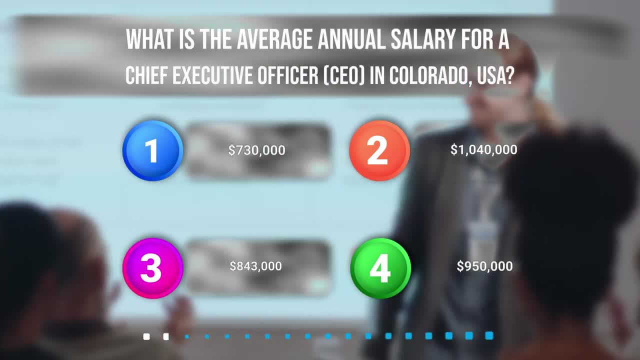 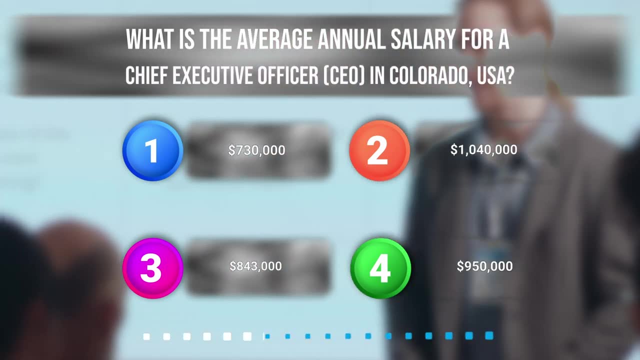 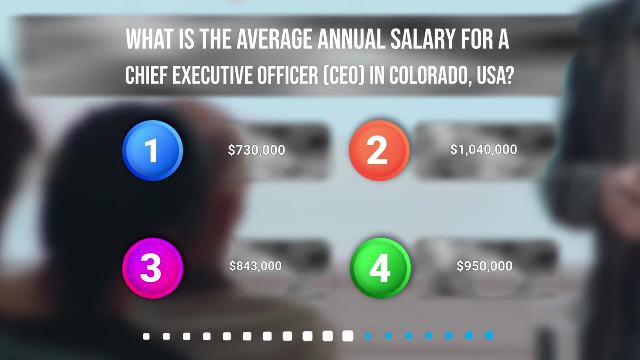 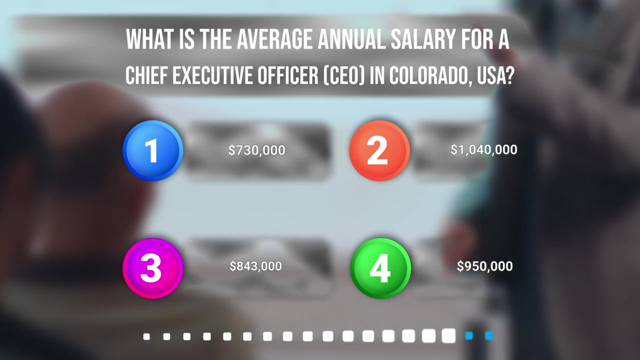 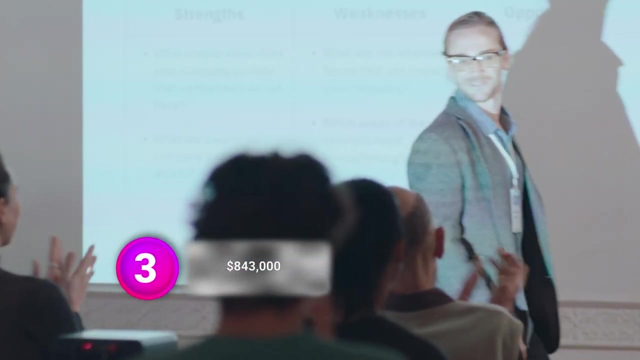 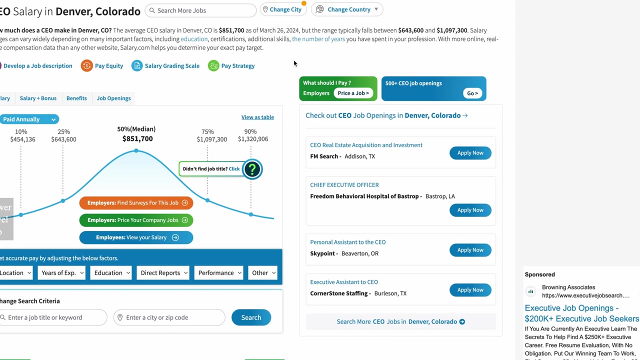 seven hundred thirty thousand dollars to one million forty thousand dollars. three eight hundred forty three thousand dollars. for nine hundred fifty thousand dollars, the answer is three eight hundred forty three thousand dollars. The average annual salary for a CEO in Denver, Colorado, is $851,700.. 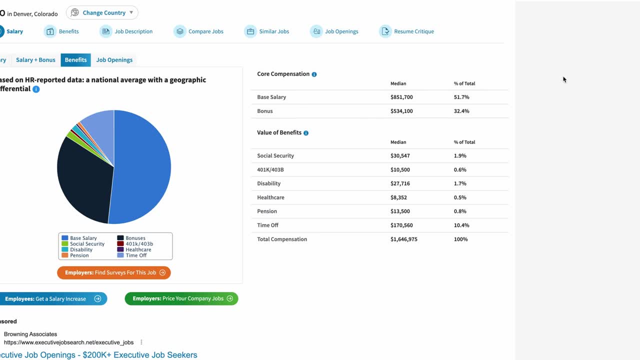 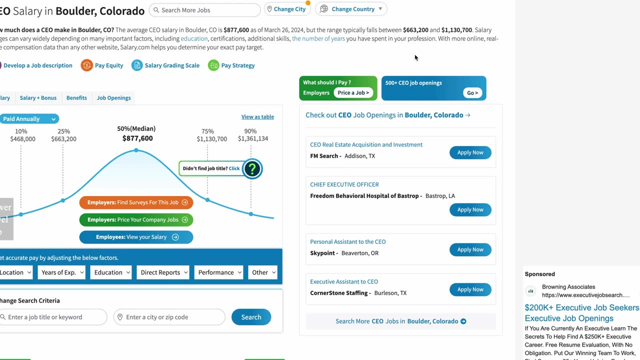 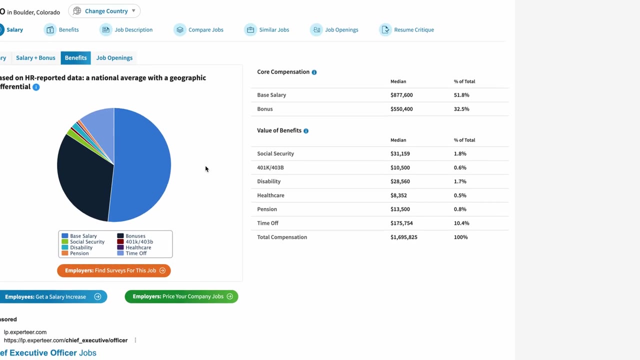 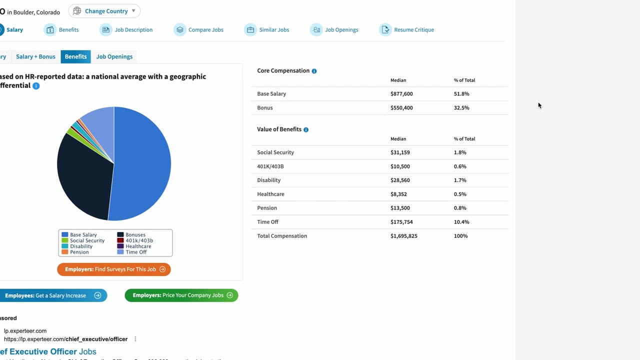 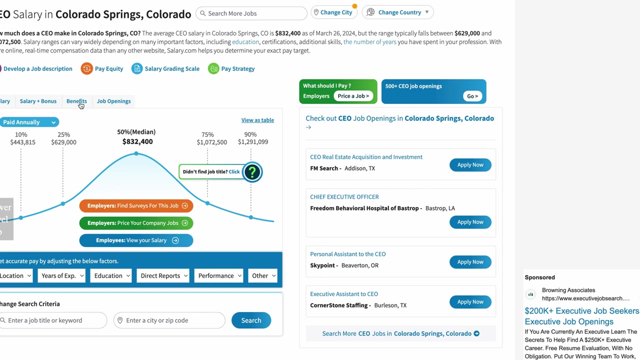 The total compensation, including all the benefits are $1,646,975.. The average annual salary for a CEO in Boulder, Colorado, is $877,600.. The total compensation, including all the benefits are $1,695,825.. The average annual salary for a CEO in Colorado Springs, Colorado, is $832,400.. 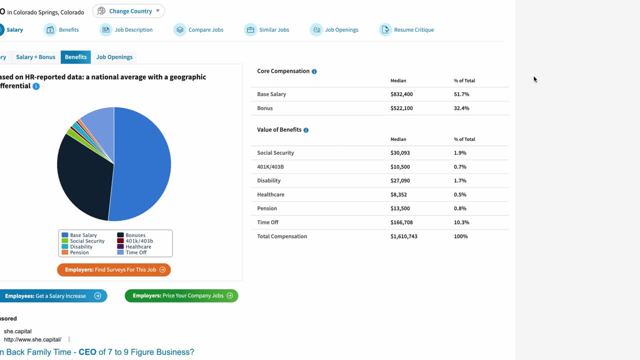 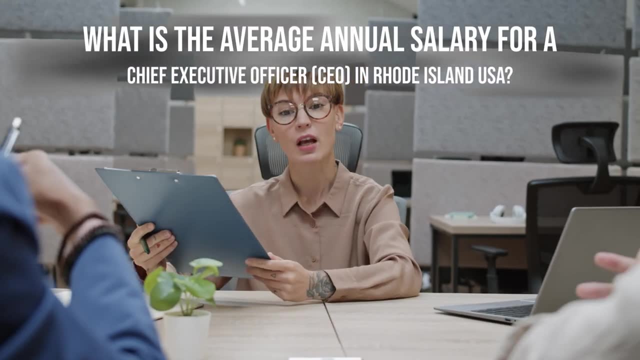 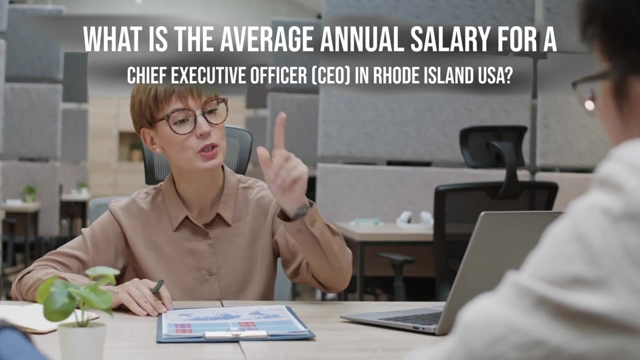 The total compensation, including all the benefits, are $1,610,743.. What is the average annual salary for a chief executive officer in Rhode Island, USA? 1. $760,333, 2. $870,500, 3. $980,000, 4. $1,090,000. 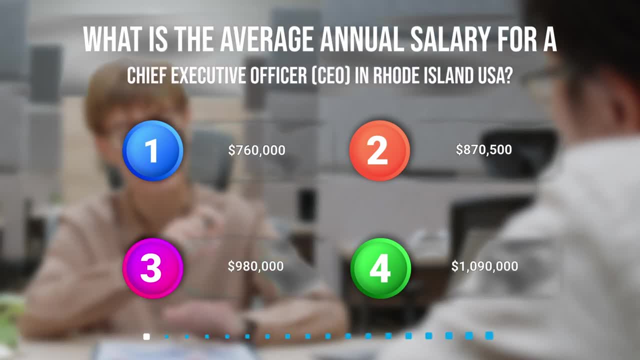 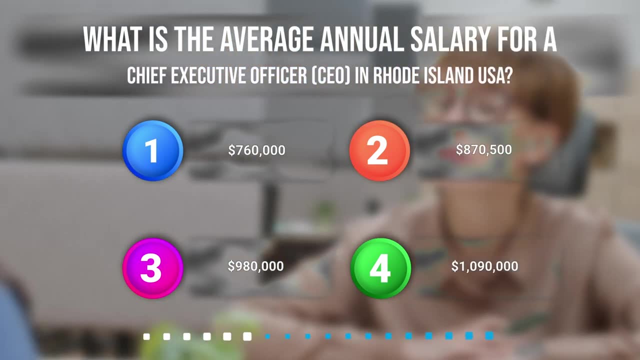 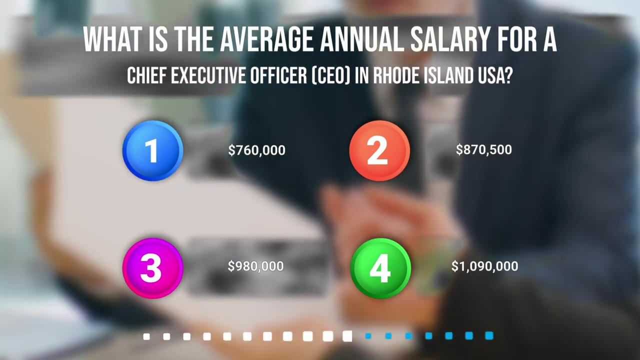 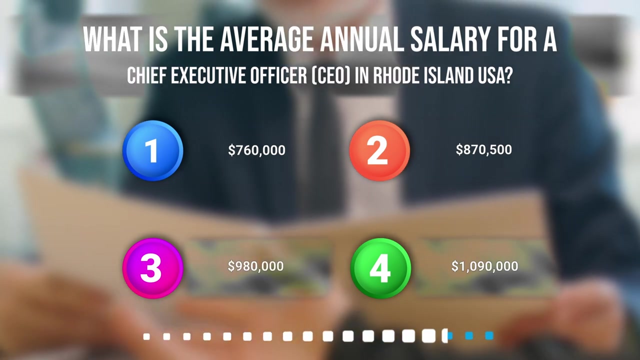 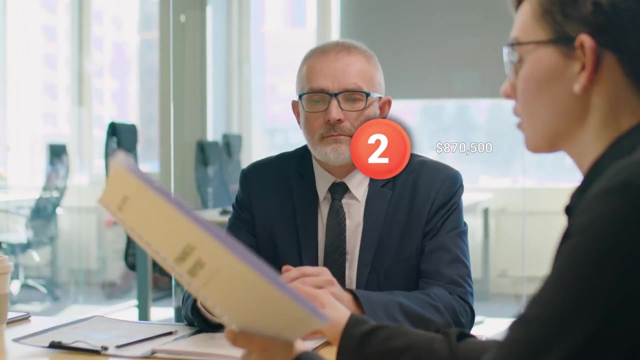 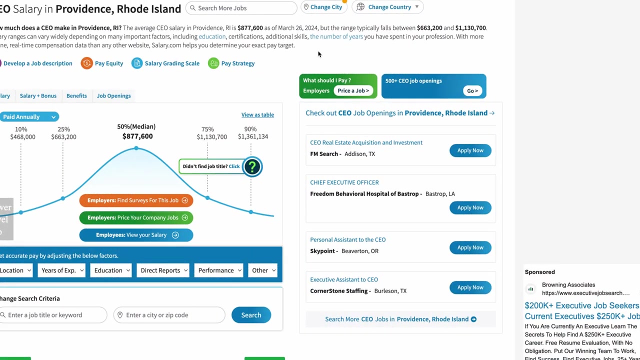 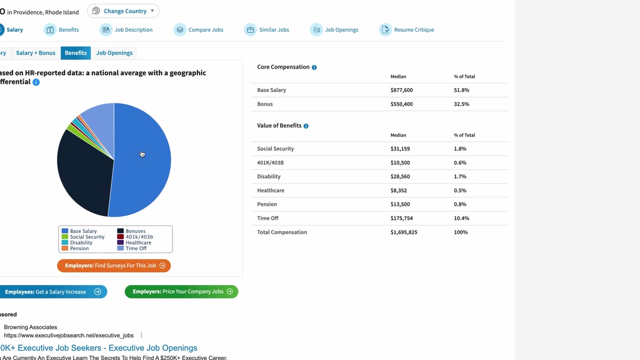 1. $760,333, 2. $870,500, 3. $980,000, 4. $1,090,000. The answer is 2, $870,500.. The average annual salary for a CEO in Providence, Rhode Island, is $877,600.